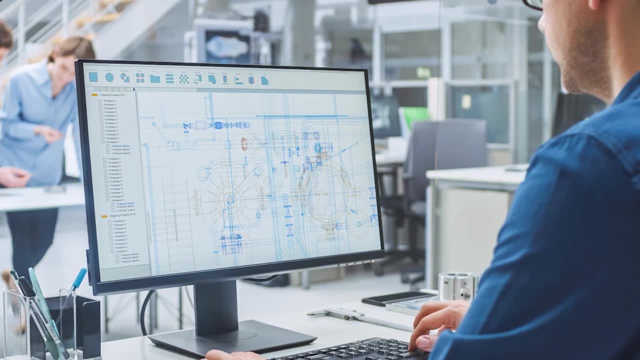 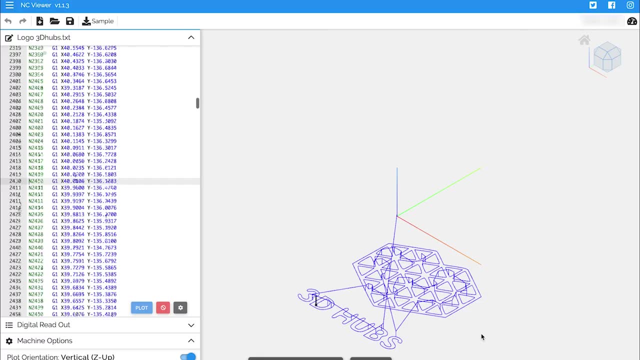 down into three steps. An engineer first designs the CAD model of the part. A machinist then turns the CAD file into a CNC program called G-code. With this G-code, the machinist sets up the CNC machining process. The CNC machinist then turns the CAD model into a CNC program called. 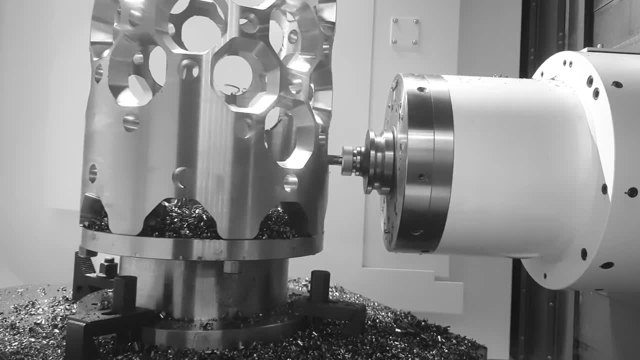 G-code. With this G-code, the machinist sets up the CNC machining process. The CNC machinist then turns the CAD model into a CNC machine. Finally, the CNC system executes all machining operations, including tool changes, cutting operations to create the part and cooling of the part and tool. 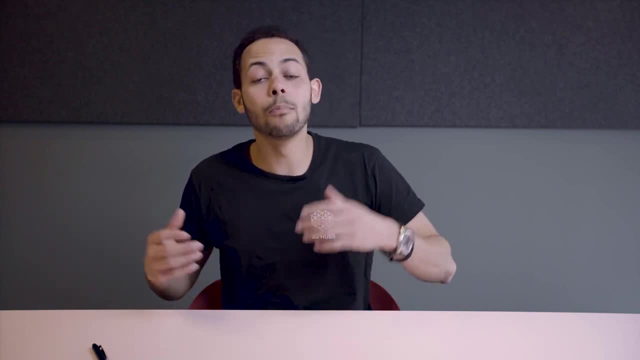 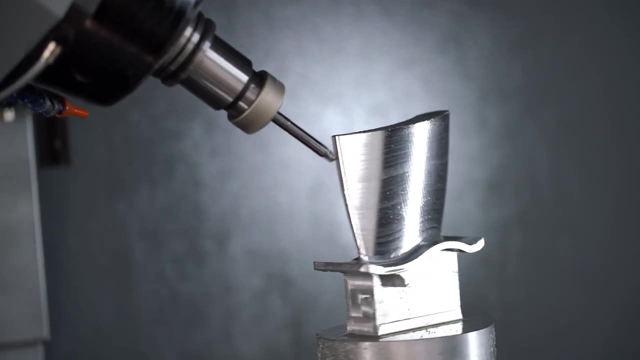 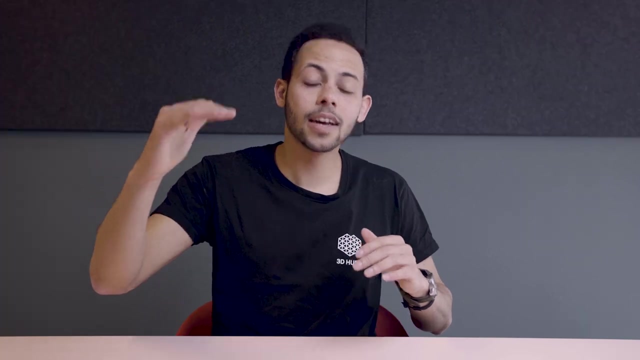 During manufacturing. CNC machining tools such as mills, lathes, grinders and routers are automated and controlled by a computer. This means that little human supervision is needed during the manufacturing process. Because of this high level of automation, CNC machining is very cost competitive or price competitive for one-off parts and medium volume production. 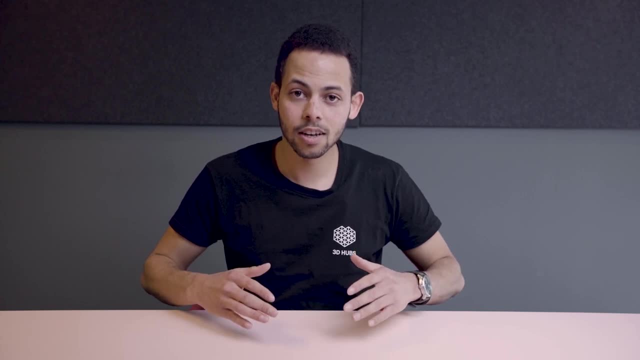 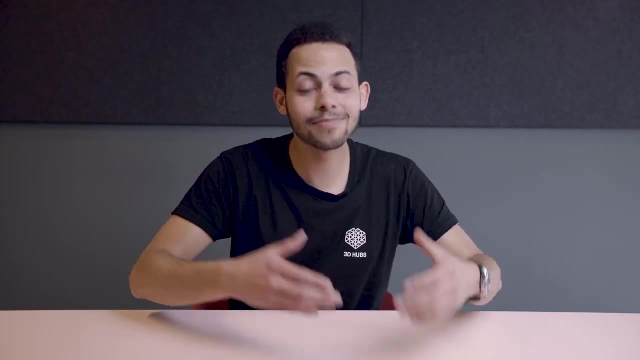 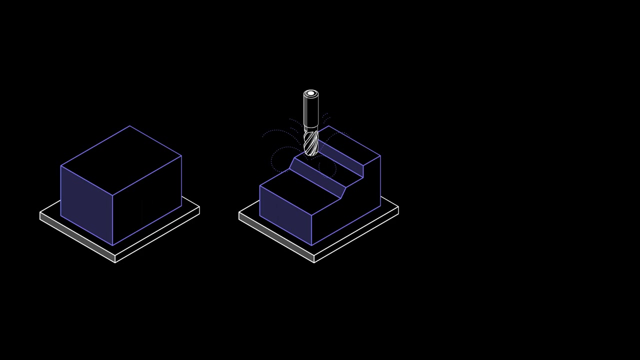 CNC machining is a subtractive manufacturing technology. This makes it fundamentally different from technologies such as 3D printing and injection molding. More on that in a bit. CNC machining is a subtractive manufacturing technology because parts are created by removing material from a solid block. This block is called the blank or workpiece. 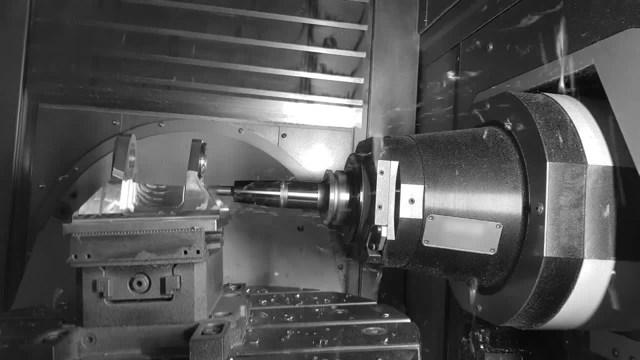 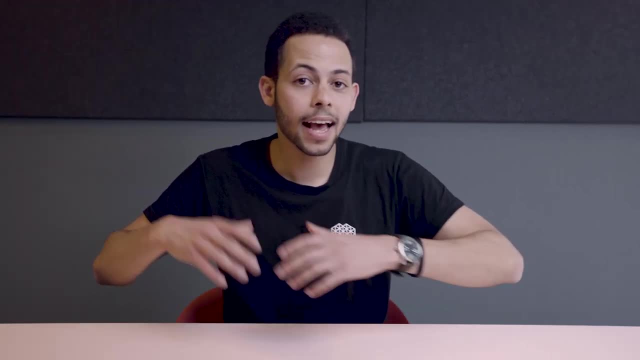 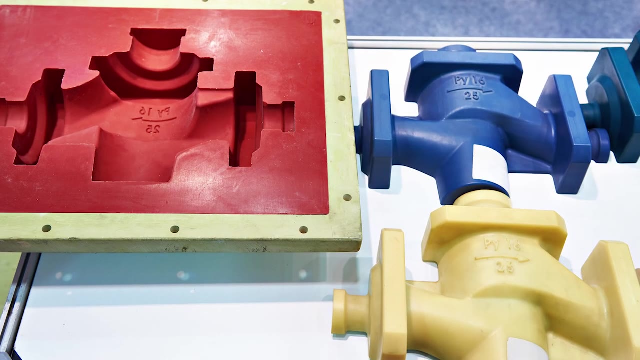 Removing material from this blank or workpiece is done by a variety of automated cutting operations. So why is CNC machining so different from 3D printing and injection molding? Well, 3D printing is an additive manufacturing technology, whilst injection molding is a formative manufacturing technology. This means that 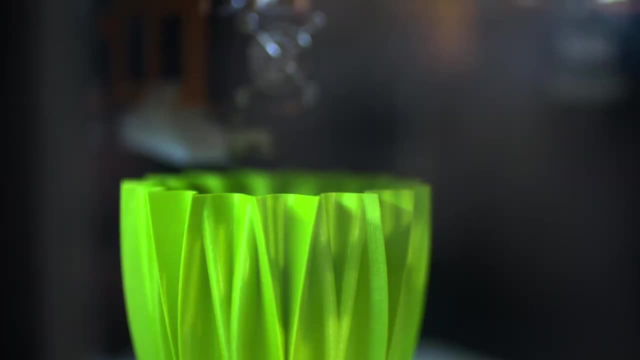 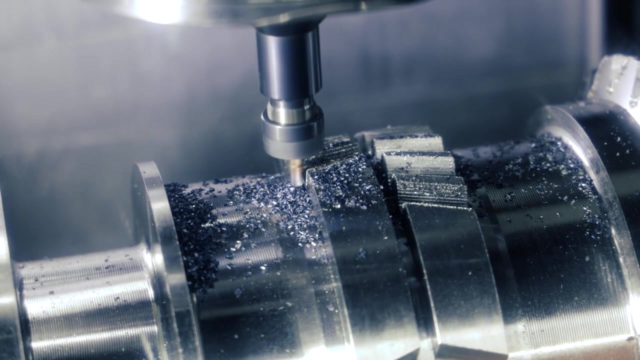 during the manufacturing process, material is added together to create parts. Quite the opposite from CNC machining. This means that the material is added together to create parts- Quite the opposite from CNC machining, Where the material is subtracted. When it comes to materials in CNC machining, 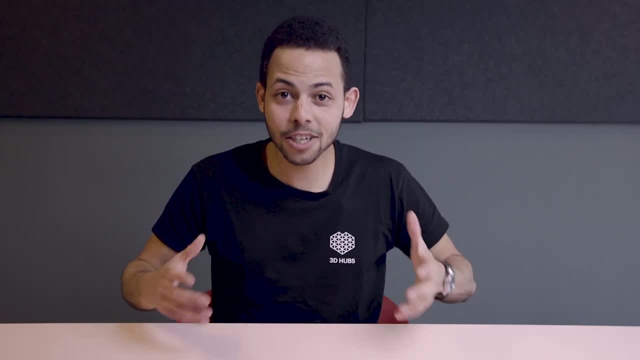 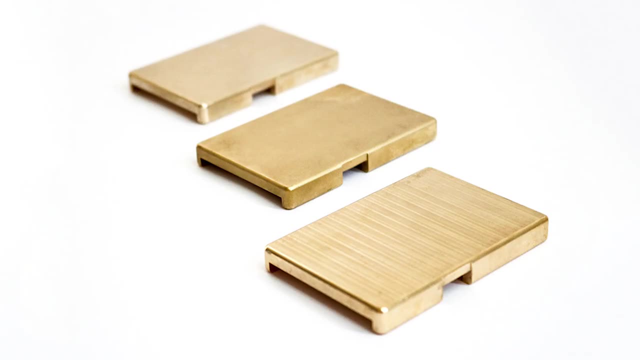 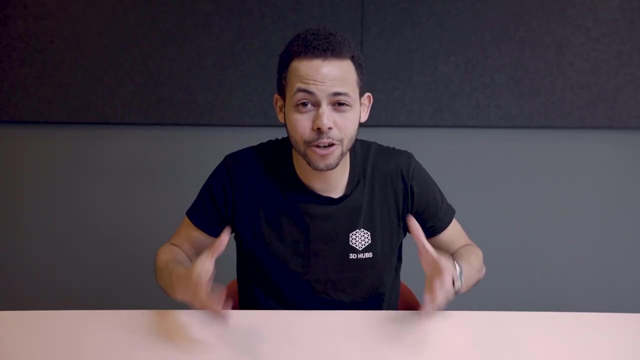 there's no shortage. Almost any kind of hard material can be CNC machined. Some of the most common materials are aluminium, brass, ABS, delrin and nylon. What CNC machining is probably best known for is its ability to create highly custom parts with tight tolerances, making it one